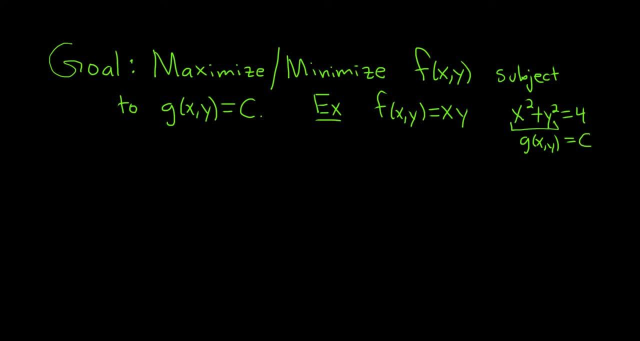 So find the maximum of x times y, subject to this condition. So these are the steps in order to do the problem. So steps, And there are some assumptions here: You have to have continuous first partial derivatives And your curve- here g of x, y equals c- has to be a smooth curve. 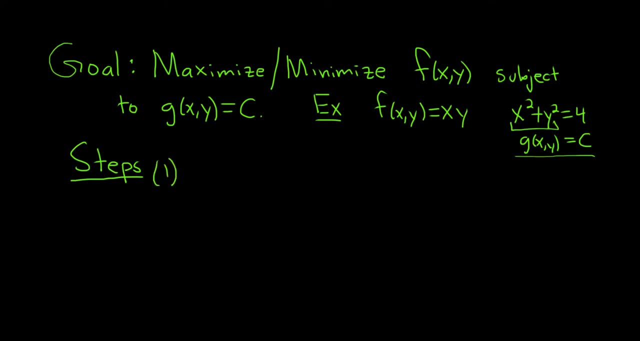 Okay. so step one in the process of Lagrange multipliers is to solve the following equations. So we have: the first equation is that the gradient of f at x, y is equal to lambda. It's the Greek letter, lambda Times the gradient of g of x, y. 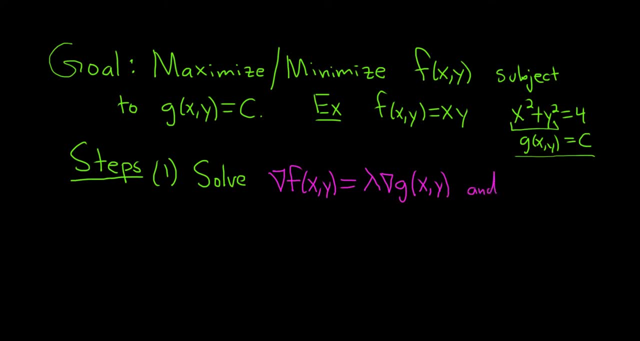 And also solve the equation g of x. y equals c. So you solve both of these equations at the same time, right, And usually it requires some algebra. It's actually pretty fun. I actually enjoy these problems quite a bit. Two: 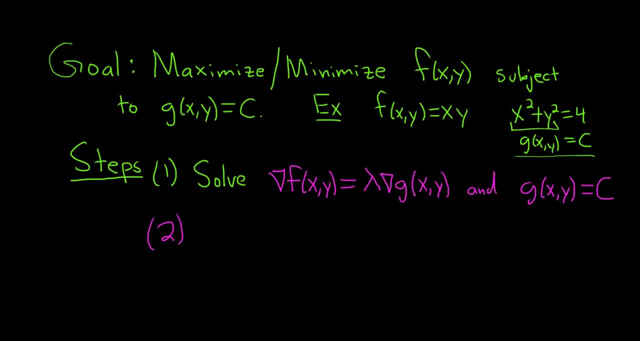 Once you get your answer or answers from the first part of the step, you plug them into your original function. So plug in, Plug in x y into f of x y And that's it. The biggest answer you get is the max. 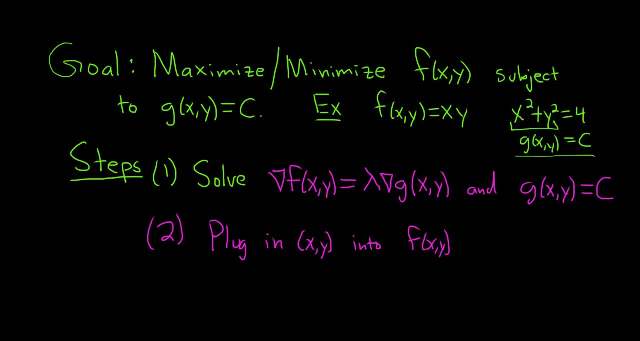 The smallest is the min. Usually you only have one. Sometimes you have a max and a min. So the biggest number you get, that's going to be your maximum, And the smallest number you get, that's going to be your minimum. 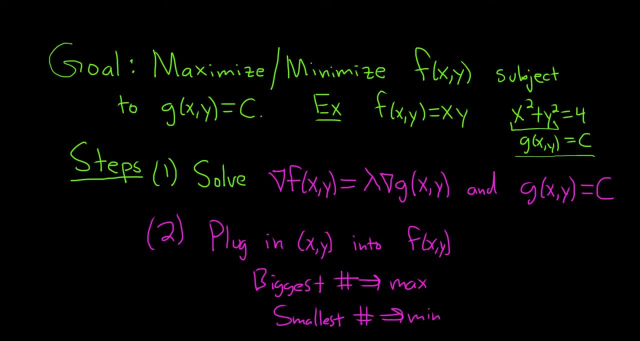 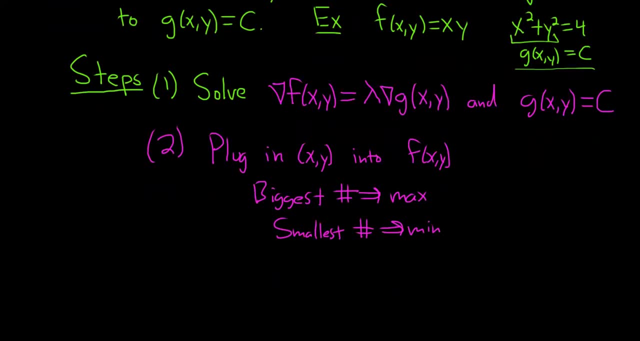 So that's how you use Lagrange multipliers. Let's do a really simple example. I have one here that looks pretty easy. Let's try it. So ex means example. Let me switch colors here. I bought something lighter, So we have f of x, y equal to x times y. 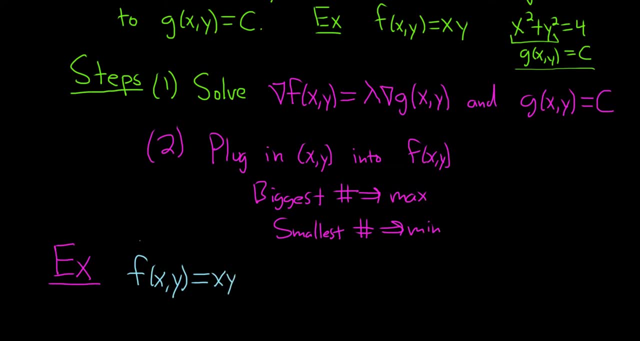 Okay, this is the function that we have, And we're asked to maximize this function. So we're going to find the maximum of this function And our constraint is x plus y, equal to 10.. That's our constraint, Okay. so first thing we have to do is compute the gradients. 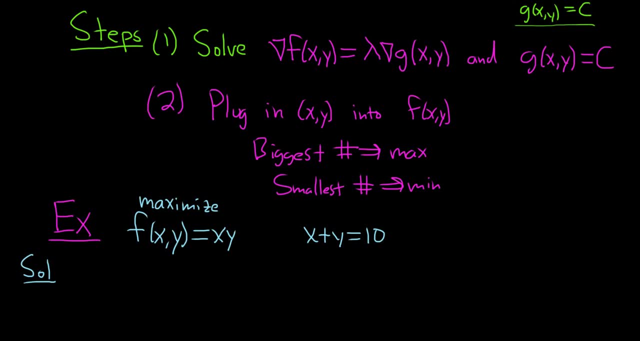 So solution. So all we have to do is use these formulas up here. So these two formulas here. So the partial derivative of f with respect to x. Well, the y is a constant right, So the derivative of x is 1.. 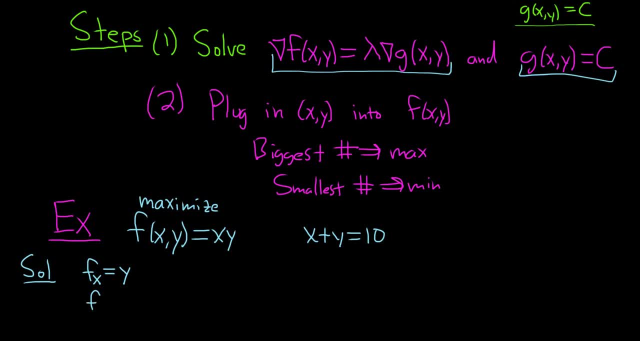 So we just get y And the partial derivative of f with respect to y. Well, the x is a constant, So the derivative of y is 1.. So we simply get x. Okay, this here is going to be our g. 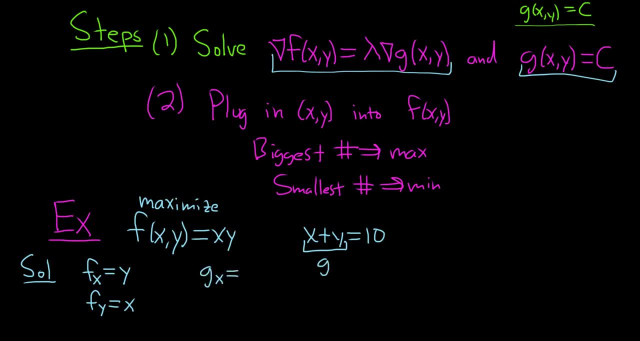 So gx is going to be equal to 1, right, Because the derivative of x is 1.. And gy is also equal to 1 because the derivative of y is 1.. Right, the other derivative, the derivative of x, is 0. 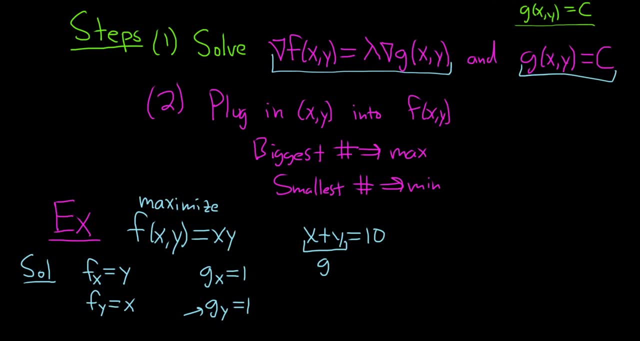 when you compute this partial, Because you treat it as a constant. Okay, so now we're good, Right? so now I'll just write the formula down. So we have gradient of f of xy That should be equal to lambda gradient of g of xy. 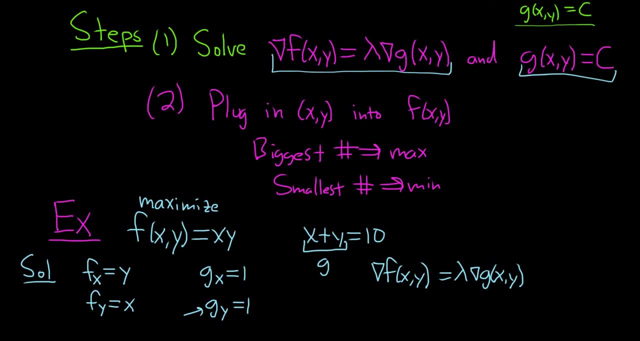 What a cool formula. Okay, and so now we simply replace this with what it is. So this is the partial with respect to x, which we said was y. So this is y, And the second component is the partial with respect to y. 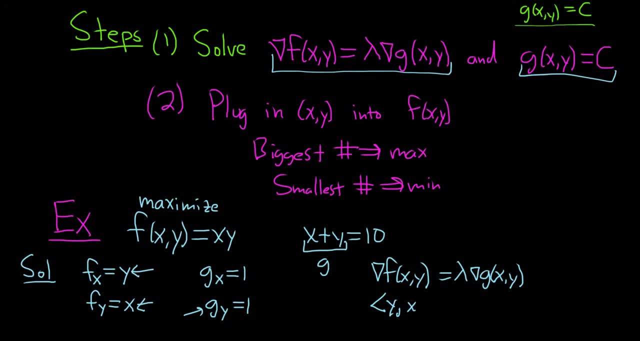 which we said was x. So x is a comma And that's equal to lambda, And these are both 1 and 1.. And we also have this condition here: x plus y equals 10.. All right, let's keep going, see what happens. 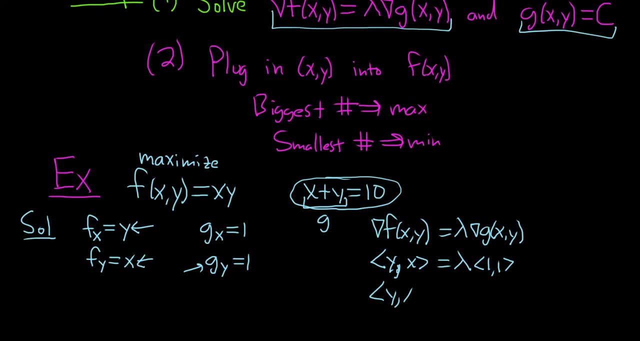 So we have y comma x equal to lambda comma lambda. So that means that lambda is equal to y And also that lambda is equal to x. All right, they're both the same right, because this means lambda is y and lambda is x. 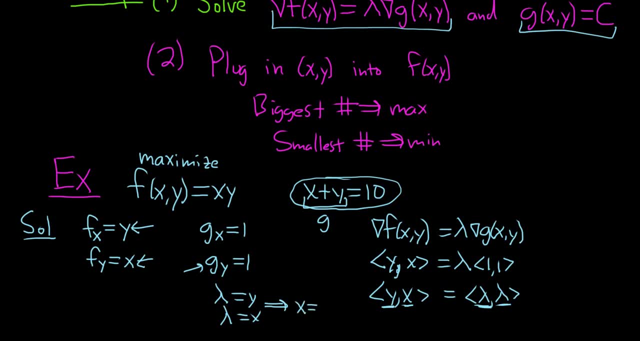 Oh, how nice. This means that x is equal to y. Okay, so we've used this condition. So now, in order to proceed in the problem, we have to use our constraint. So that's this condition up here. So we're told that x plus y is equal to 10..